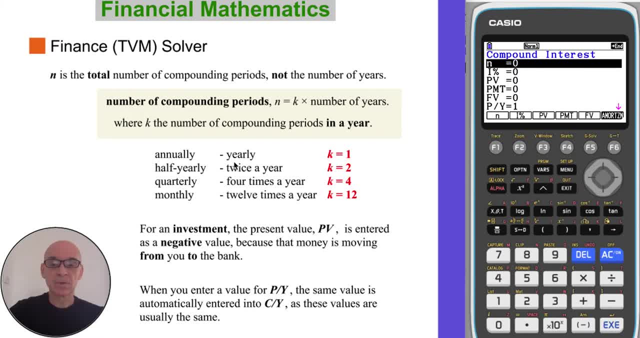 And if the interest is compounded annually or yearly, then K is equal to 1.. If the interest is compounded half-yearly, that's twice a year, then K is equal to 2.. If the interest is compounded quarterly, that's 4 times a year, then K is equal to 4.. And if the interest 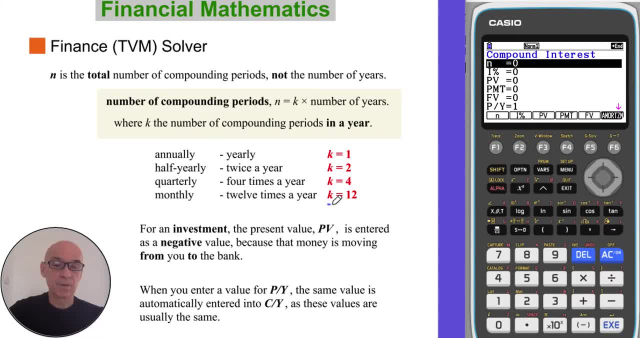 is compounded monthly- that's 12 times a year- then K is approximately over 3.. And from the original formula you can see that thebagging returns are much better at compounding is equal to 12.. For an investment, the present value P of E is entered as a negative value. 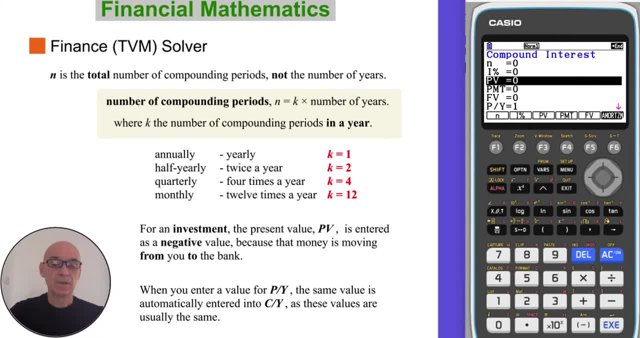 because that money is moving away from you into the bank. for example, When you enter a value for P slash Y, the number of payments per year, the same value is automatically entered into C slash Y, the number of compounding periods per year, as these values 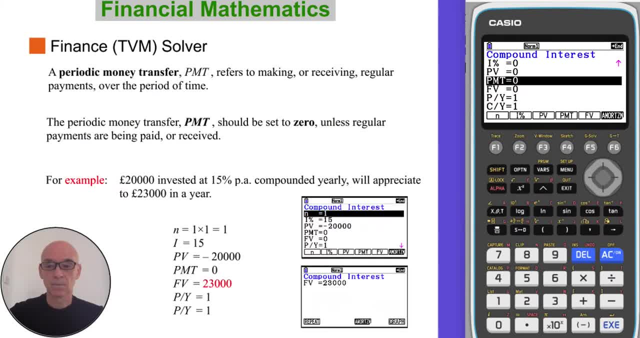 are usually the same. A periodic money transfer- PMT refers to making or receiving regular payments over the period of time. The periodic money transfer should be set to zero unless regular payments are being paid or received. When solving compound interest problems using the Finance. 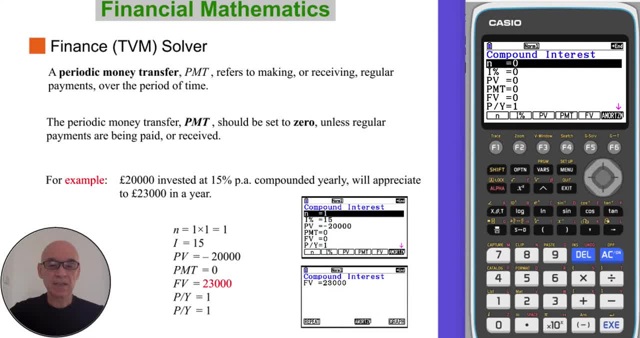 Solver app, your method should be to write down the values of the six variables that you enter into the calculator, as shown in this example here. For the total number of compounding periods, you can either enter 1 times 1 or simply enter 1.. For the interest rate: enter: 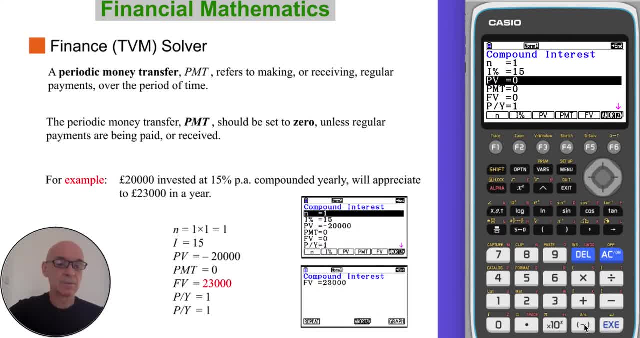 15.. For the present value, as it's an investment, you enter negative 20,000.. As there are no periodic money transfers, we set the PMT to equal zero. We will leave the future value, FV, blank, as that's what we're going to solve for, And then we set the payments per year and 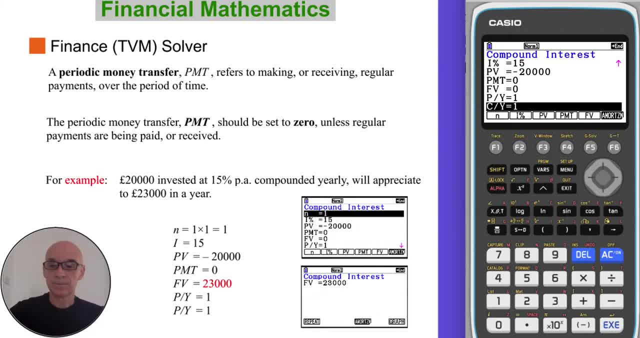 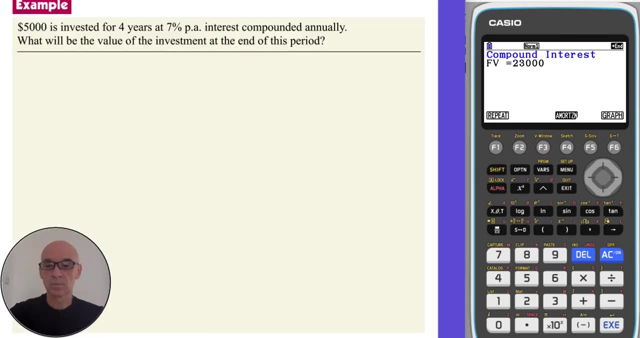 the future value as: 1. To solve for the future value FV, we press F5,, giving a future value of 23,000 pounds after one year. In this question we're asked to find the value of the investment at the end of the four year period. So to repeat a calculation, we start by pressing. 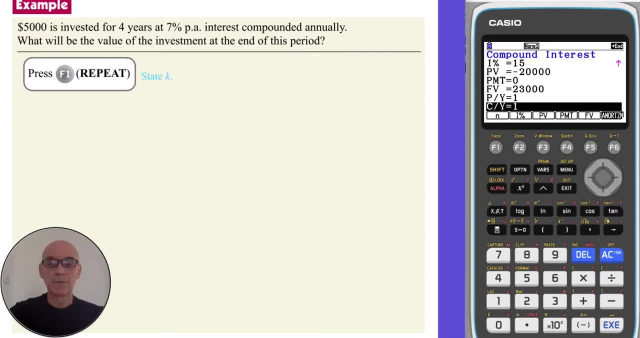 F1. If we first state K, the number of compounding periods per year, and as the interest is compounded annually, then K is equal to 1.. Then if we find N, the total number of compounding periods, So compounding once per year for four years 1 times 4 is equal to 4.. And again you can. 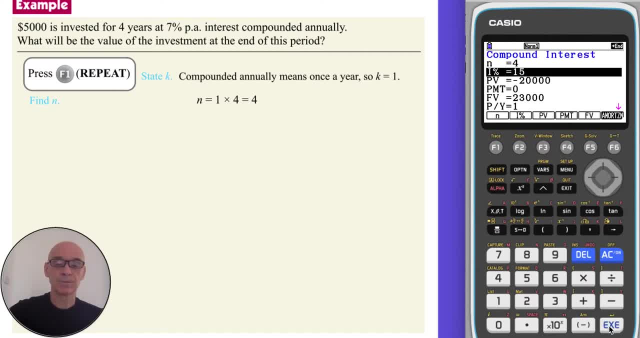 either enter 1 times 4 or simply enter 1.. Next state the interest rate, which is 7.. Then state the present value and, as it's an investment, that's equal to negative 5,000.. As there are no periodic monthly transfers, 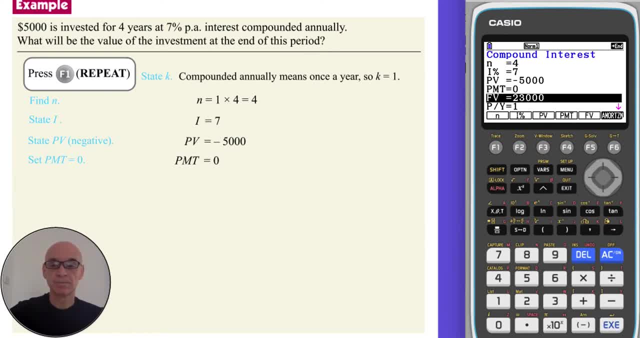 then set PMT equal to zero. As we're going to solve for the future value FV, you can either leave the previous value there or you can set FV equal to zero, Setting the payments per year and the number of compounds. 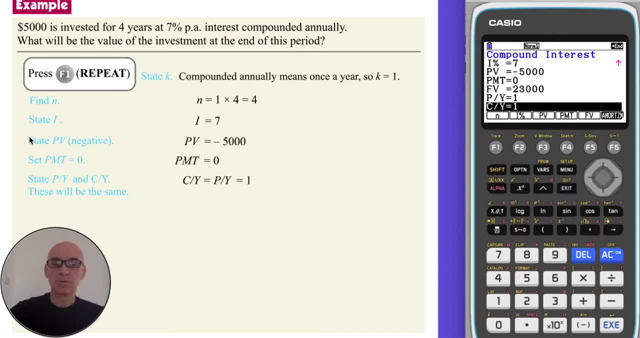 per year equal to 1, as K was equal to 1.. In other words, the interest was compounded annually. To solve for FV, we press F5, and as the interest is compounded annually, then K is equal to 1.. 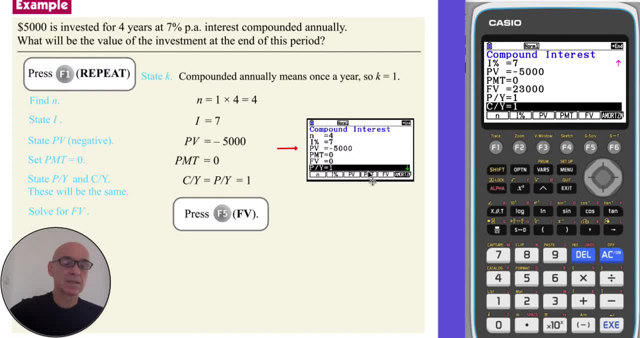 To solve for FV, the future value, we press F5,, given the value shown, And since it represents money, we should give the answer correct to two decimal places. So the investment will amount to $6,553.98 after four years. 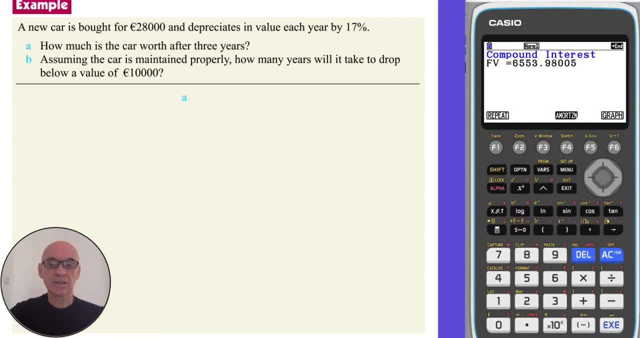 In part A of this question we're asked to calculate the value of the car three years after it was purchased. So pressing F1 for a repeat calculation, starting by stating K the number of compounds per year, and since depreciation is annual, K is equal to 1.. And then finding N, the total. 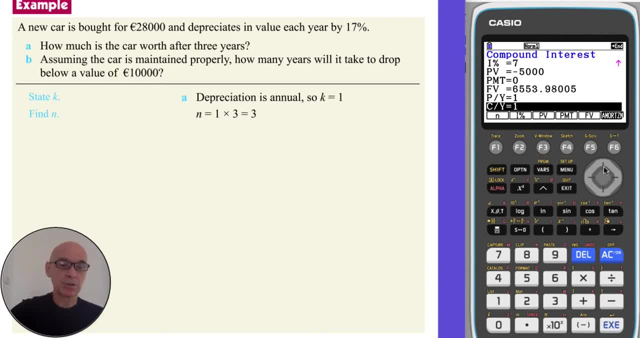 number of compounding periods, That's one depreciation for each of three years. So 1 times 3 is equal to 3, so it either N times 3 or simply N times 3.. Next stating I: and since it's depreciation, it will be entered as negative 17.. 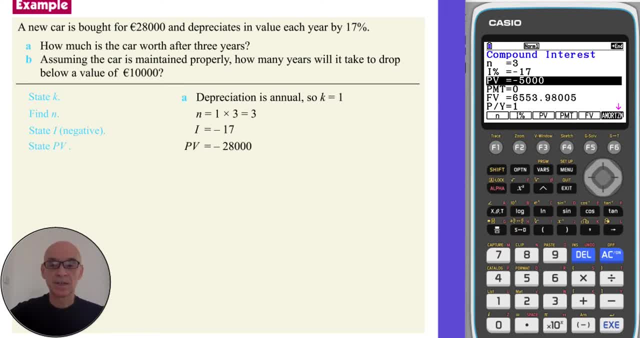 Next stating PV, the present value. And since the car will be small, it will be equal to N. So this is the current value of the present value And we're going to continue after the was purchased for 28,000,. again, that's money going away from you, so you enter that as. 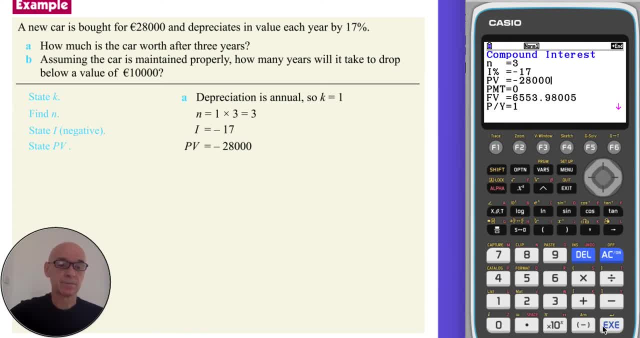 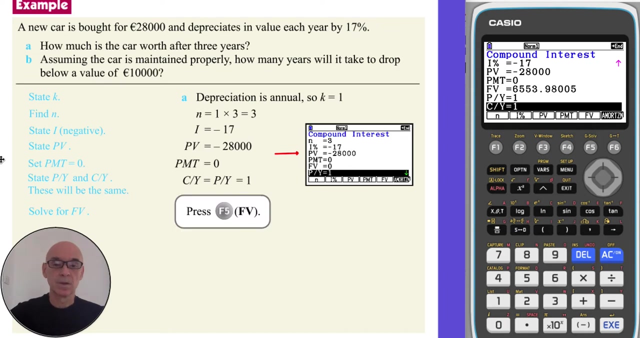 negative 28,000.. There are no periodic money transfers. so set PMT equal to zero, Set in payment per year and number of compounds per year both equal to one as its depreciation, which is annual. To solve for FV, a future value, we press F5, giving the value shown. 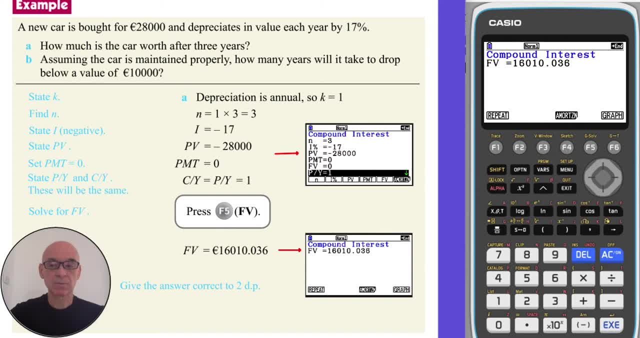 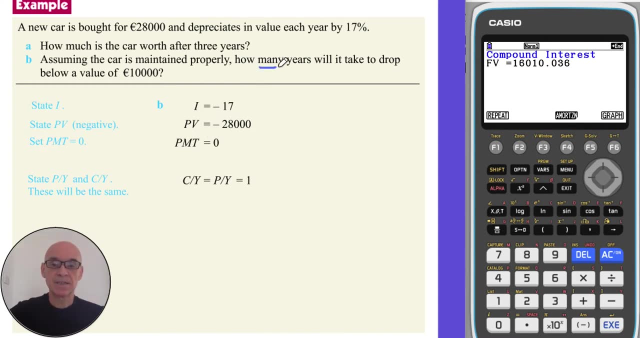 Again rounding the amount correct to two decimal places. So after three years the value of the car is zero. The future value is 16,010 euros and four cents. In part B we're asked to find how many years it will take for the value of the car to drop below 10,000 euro. So again, pressing. 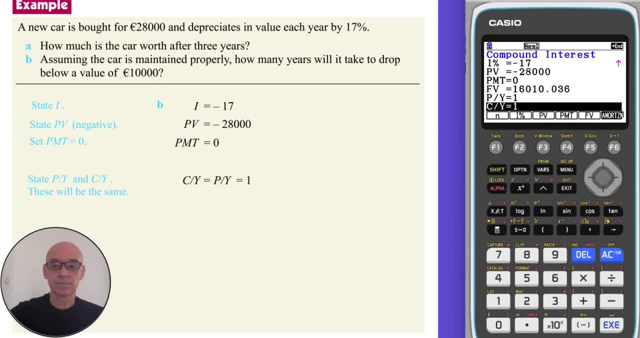 F1 for a repeat calculation, and much of the information remains the same. We just need to set the future value. This value will be divided by F4.. Now to solve for N, the number of compounded periods, Press F1.. 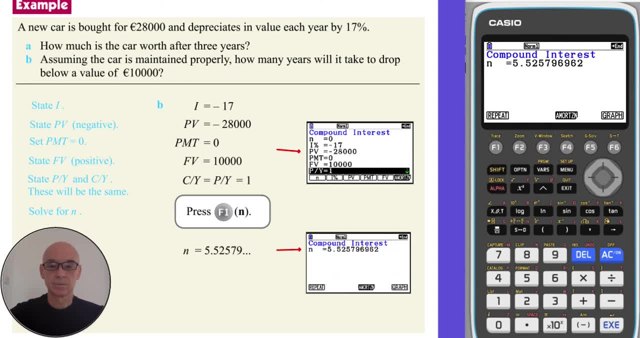 Even the value shown Now as K is equal to one. the number of compounded periods is also equal to the number of years. So, rounding up to the next whole year, it will take 6 years for the value of the car to drop below. 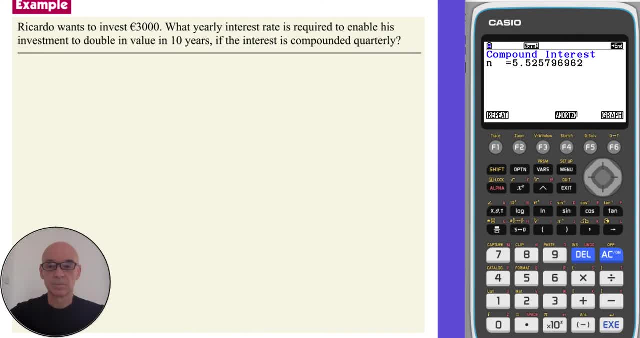 10,000 euro. In this question we have to find the yearly interest rate required to enable Ricardo's investment of 3,000 to double in 10 years. So pressing F1 for a repeat calculation, finding k the number. 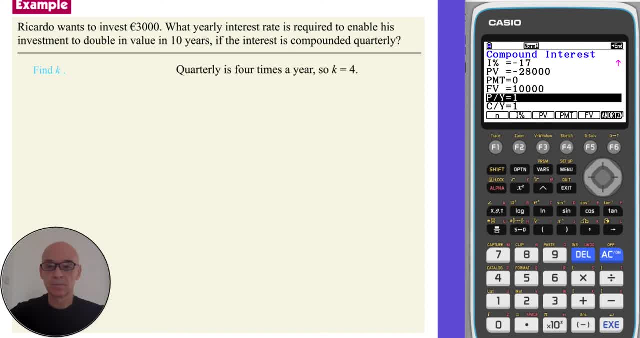 of compounded periods per year, and since the interest is compounded quarterly, then k is equal to 4.. Next, stating the total number of compounded periods so 4 times per year, over 10 years will be 40. So we can either type in 4 times 10,. 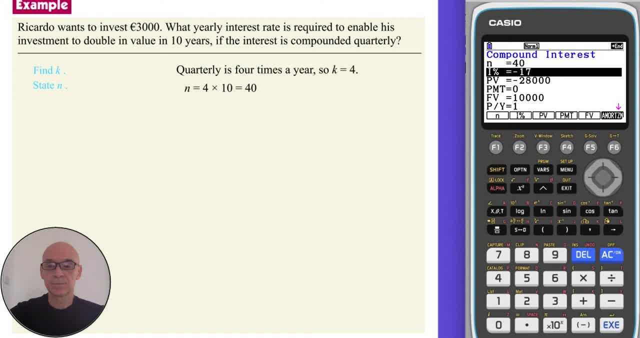 or you can enter 40.. Now, since we want to solve for i the interest rate, you can either just ignore the previous value or you can enter it as 0.. Stating the present value pv as negative 3,000, since it's an investment. 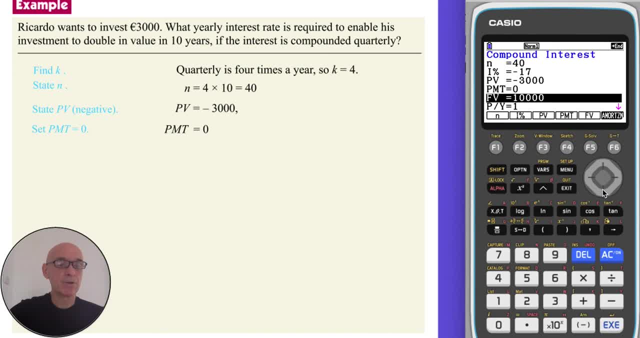 Setting pmt equal to 0,, as there are no periodic money transfers. Finding the future value and double 3,000 is equal to 6,000.. So we enter 6,000.. Stating the payments per year and the number of compounds per year. 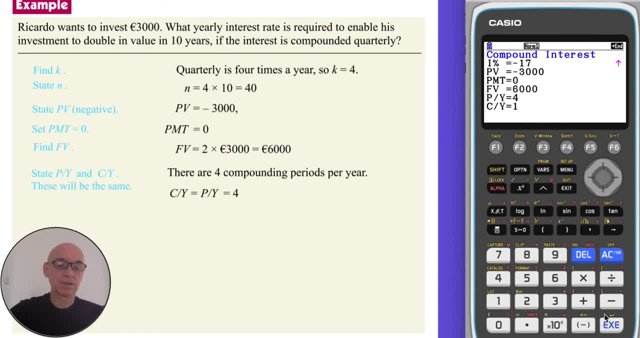 is equal to 4, as it was compounded quarterly. So we enter 6,000.. And to solve for, i press F2.. And to solve for, i press F2.. And to solve for, i press F2.. 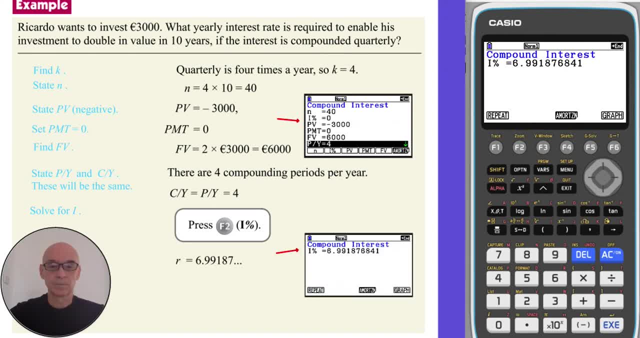 Keeping the value shown. Keeping the value shown, Rounding into three significant figures. the interest rate required is 6.99%. The interest rate required is 6.99%. In this question we're asked to find how much Ivana needs to invest.